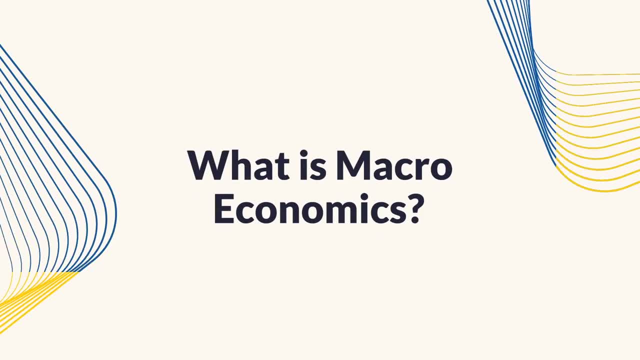 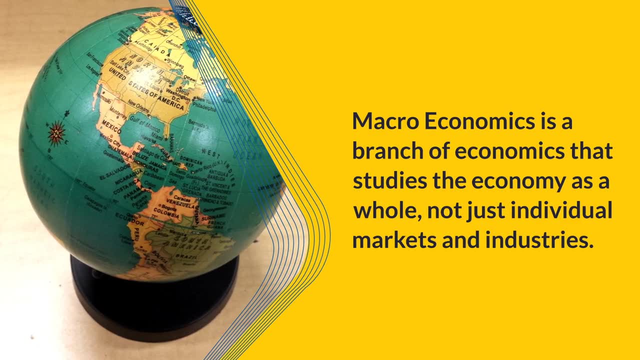 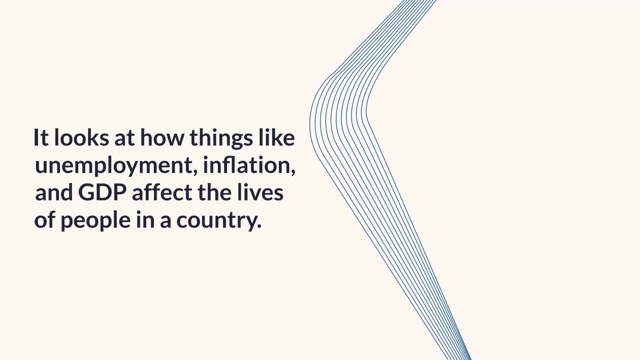 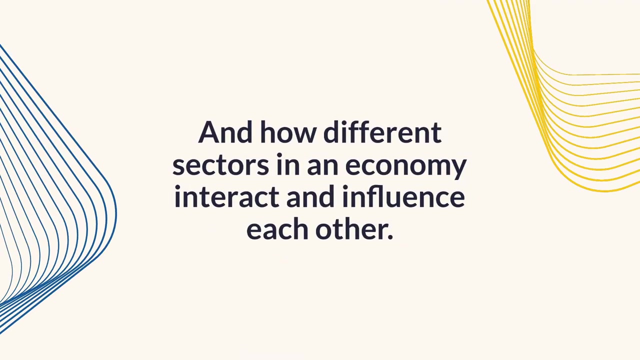 What is macroeconomics? Macroeconomics is a branch of economics that studies the economy as a whole, not just individual markets and industries. It looks at how things like unemployment, inflation and GDP affect the lives of people in a country and how different sectors in an economy interact and influence each other. 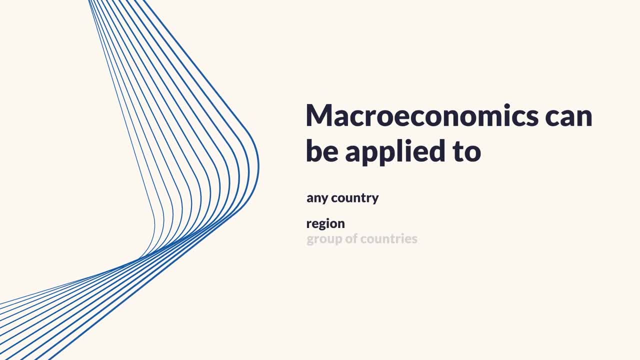 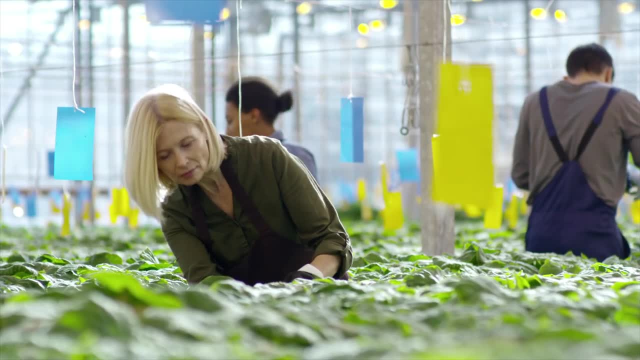 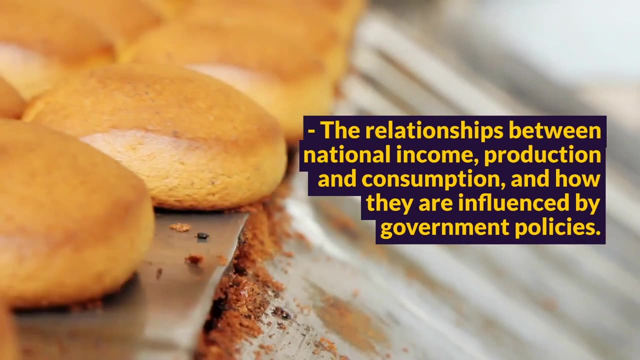 Macroeconomics can be applied to any country, region or group of countries. Some of the topics studied in macroeconomics are: the relationships between national income, production and consumption and how they are influenced by government policies. The effect of international trade on macroeconomic variables. 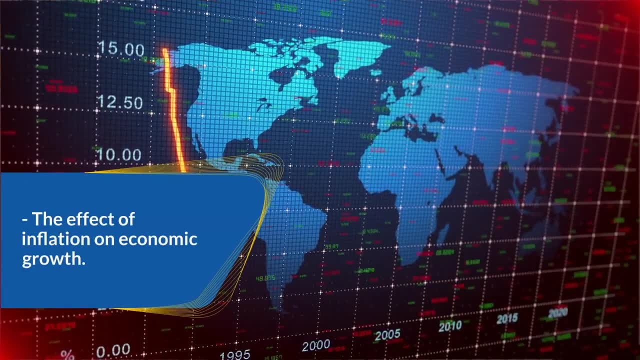 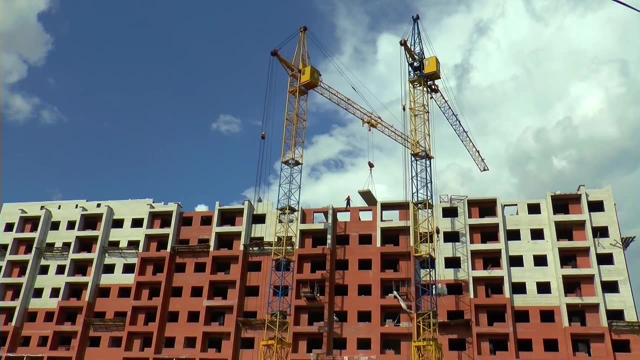 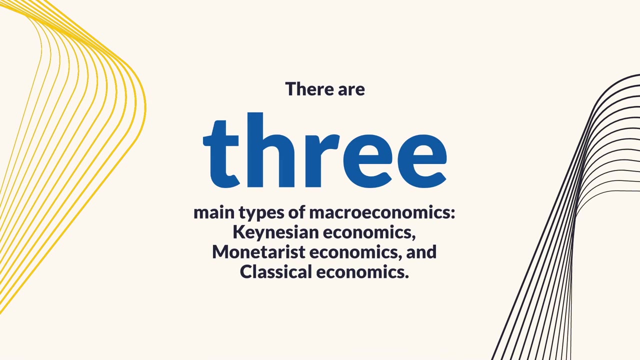 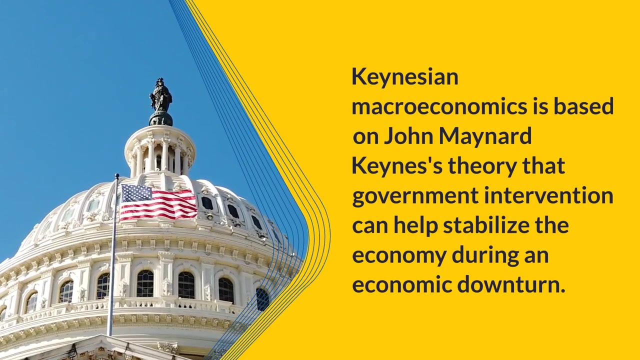 such as employment, wages and prices And the effect of inflation on economic growth. There are three main types of macroeconomics: Keynesian economics, monetarist economics and classical economics. Keynesian macroeconomics is based on John Maynard Keynes' theory. 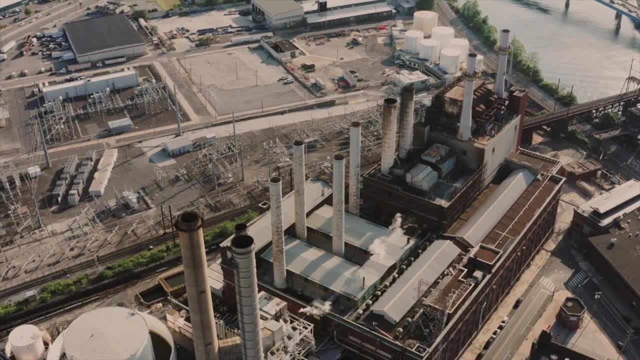 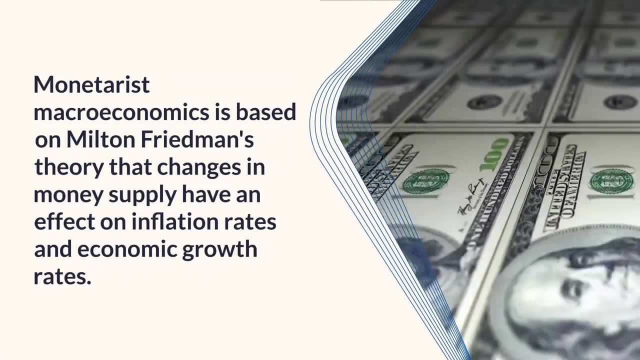 that government intervention can help stabilize the economy during an economic downturn. Monetarist macroeconomics is based on Milton Friedman's theory that government intervention can help stabilize the economy during an economic downturn, And it is based on the theory that changes in money supply have an effect on inflation rates and economic growth rates. 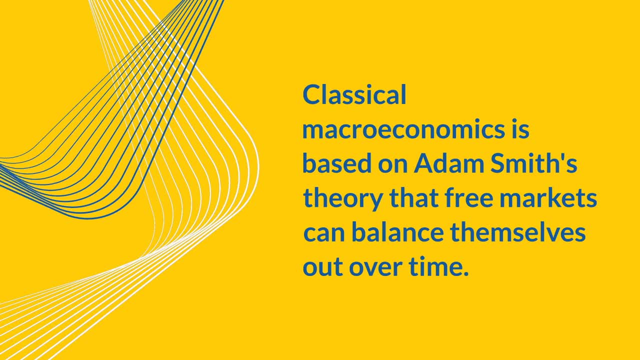 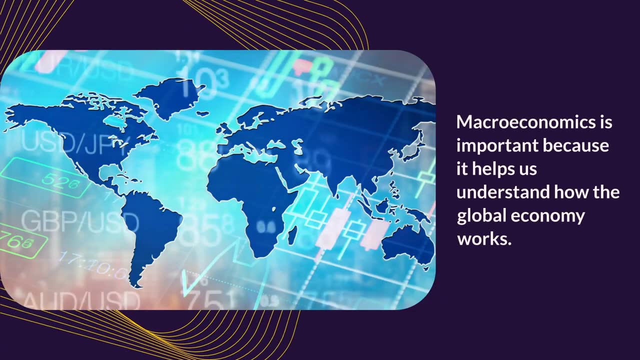 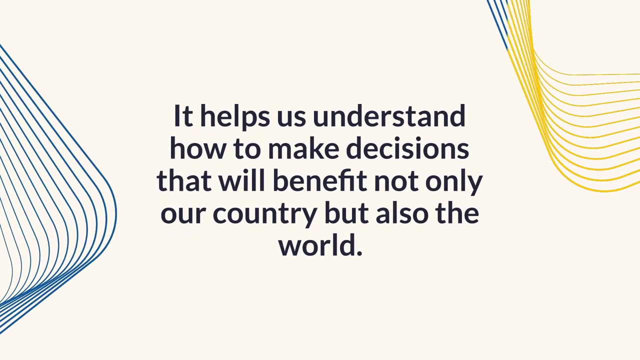 Classical macroeconomics is based on Adam Smith's theory that free markets can balance themselves out over time. Macroeconomics is important because it helps us understand how the global economy works. It helps us understand how to make decisions that will benefit not only our country, but also the world. 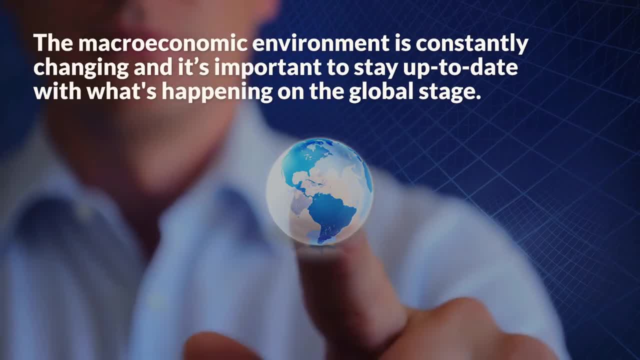 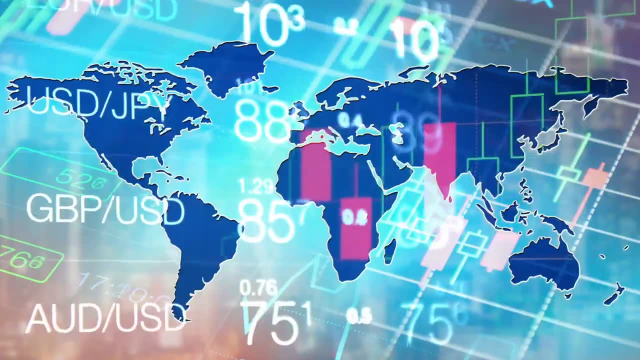 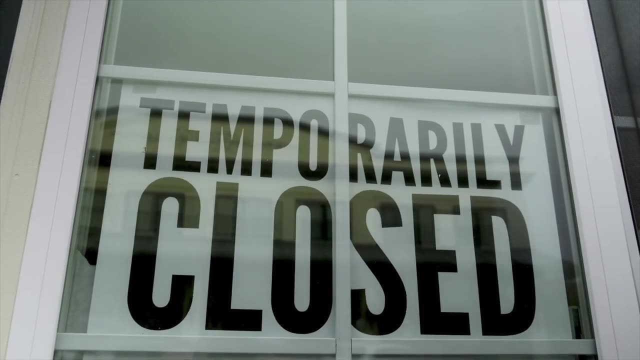 The macroeconomic environment is constantly changing and it's important to stay up to date with what's happening on the global stage. You don't want to find out that your business has been negatively impacted by a change in policy at a later date, after it's too late. 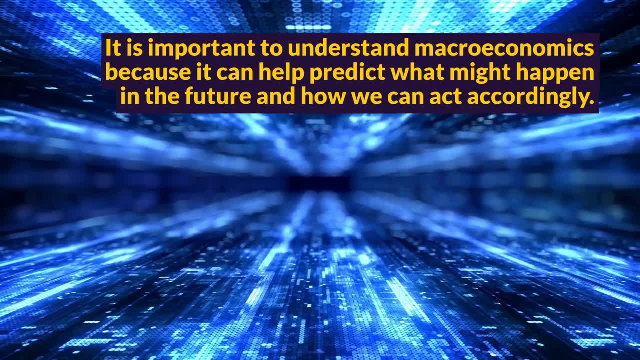 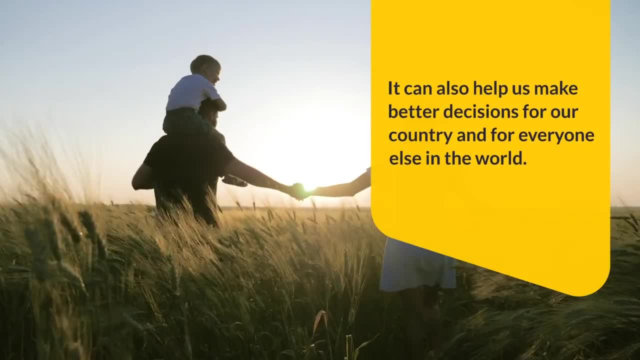 It is important to understand macroeconomics because it can help predict what might happen in the future and how we can act accordingly. It can also help us make better decisions for our country and for everyone else in the world.